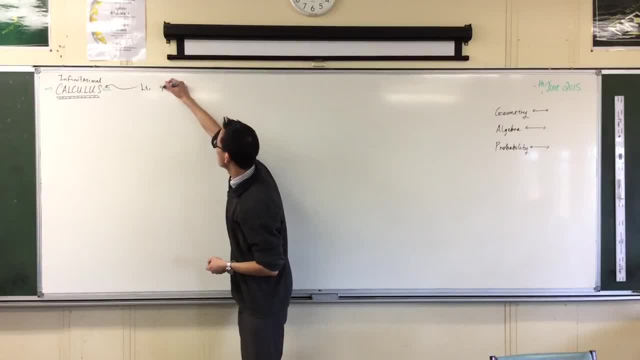 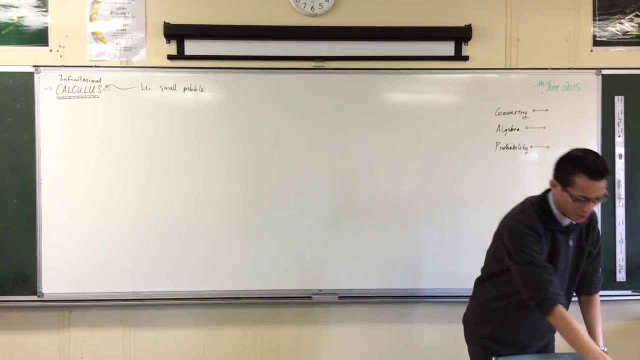 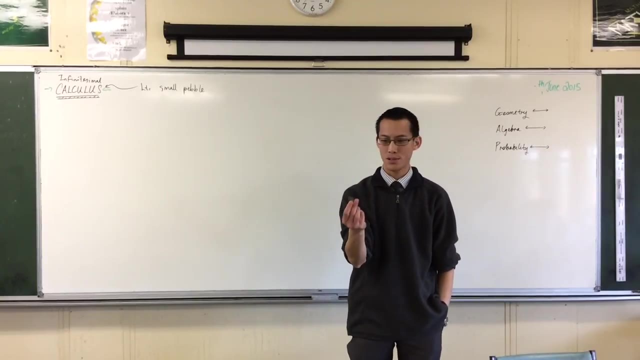 it means: um, it's Latin for small pebble- and you're like: what does? what? does that have to do with anything? And um, there goes my small pebble, Small pebbles. small pebbles are what were used to calculate with in the early days in ancient Rome, right, 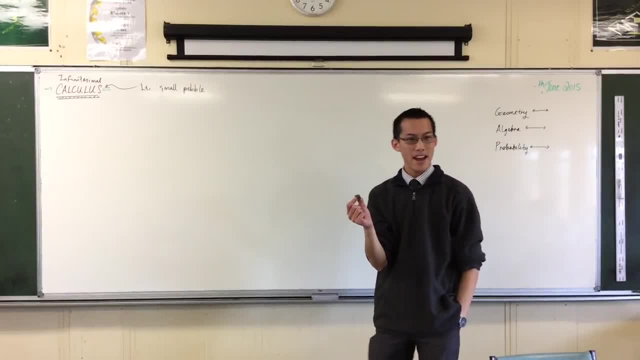 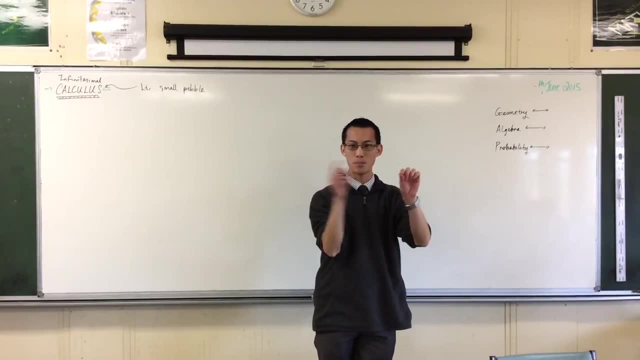 They get a whole bunch of a whole bunch of small pebbles, right, And some, um, some smart guy in some, some country, I don't know its name, puts all these pebbles on like rows and move them around and call them abacus. okay. 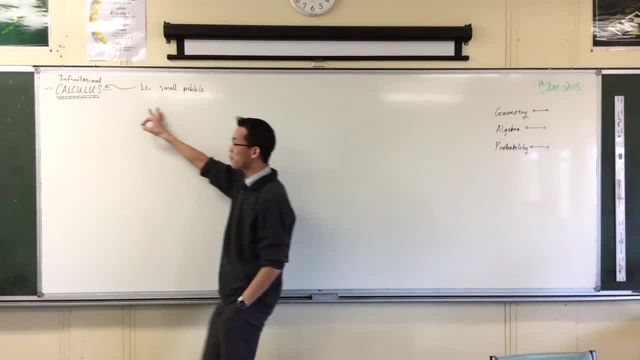 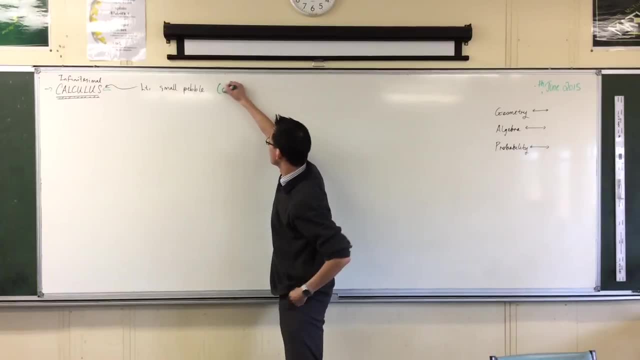 Small pebbles are what are used for, for counting and for calculations, right, By the way, it's also where we get the same word: chalk, chalk, calc. you get it, And, in fact, if any of you ever become, 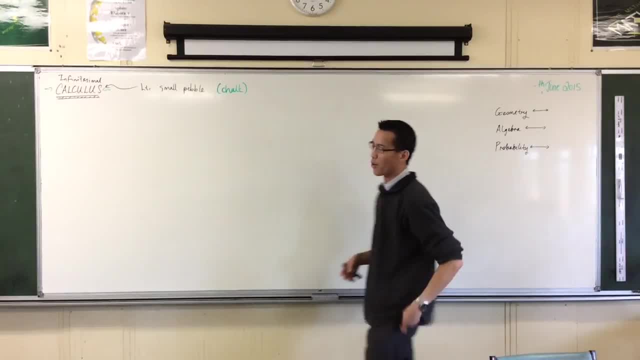 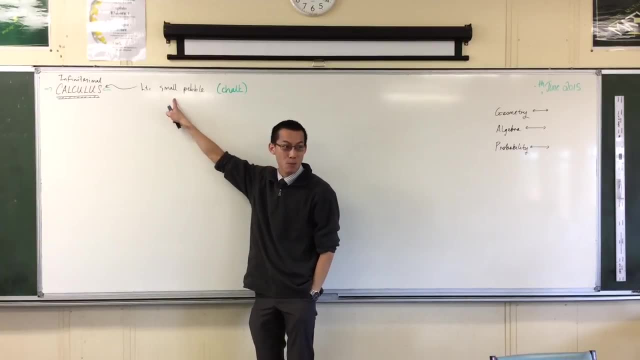 calcium. that's exactly right. if any of you become dentists or or go to the dentist, they might say: oh, you have calculus on your teeth, which, by the way, not a good thing, because you're not meant to have small pebbles on your teeth Like it's a, it's a, it's a. 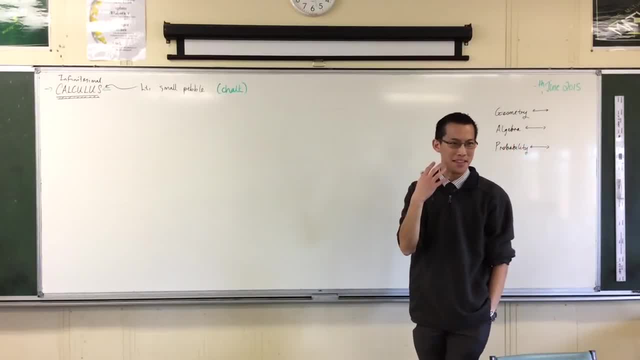 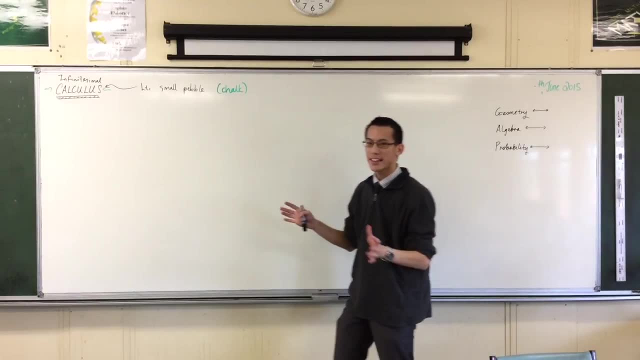 you know all of the um, gross stuff which is not meant to be there and it's damaging your teeth. okay, So calculus, right, It's really this word for calculation- and the fact that it took over, like what we're about to do, this little subtopic. 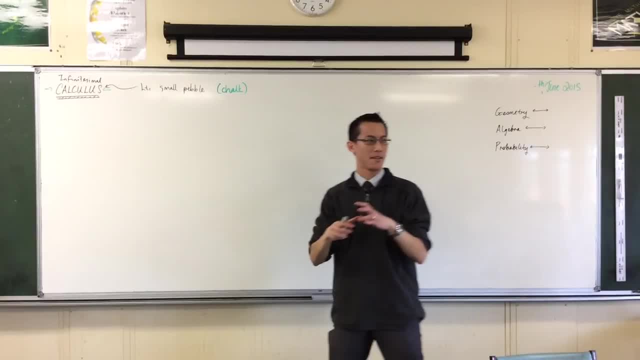 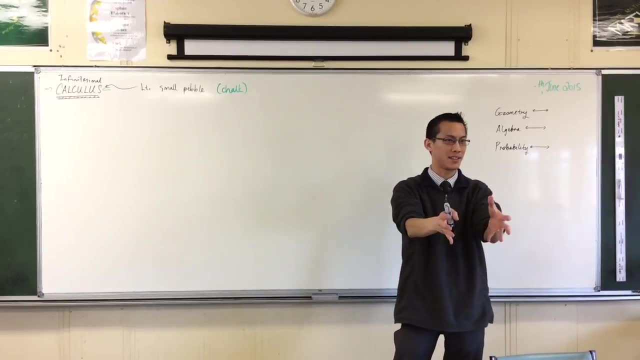 it took over from like: can you imagine, like: okay, mathematics is a really, really big word, right. And if just one little topic in mathematics became called mathematics, right? What does that say about all of the other things? right? 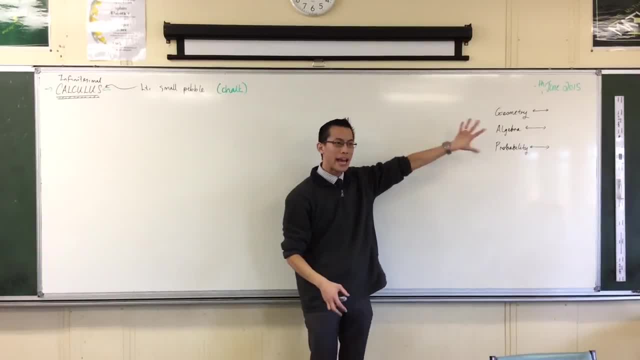 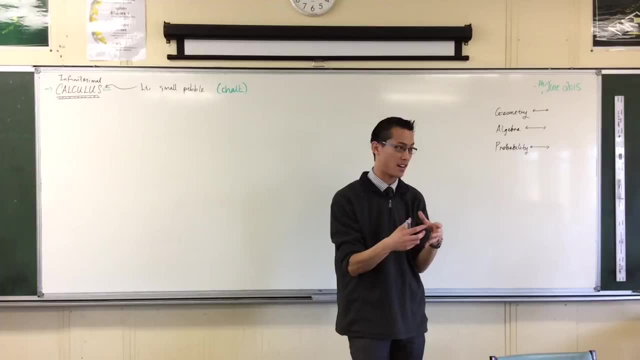 It says like this is really, really important. We have many branches of mathematics, right, Calculus is just one of them. Each of them is is sort of keyed into one single big idea. okay, You think about this with me. 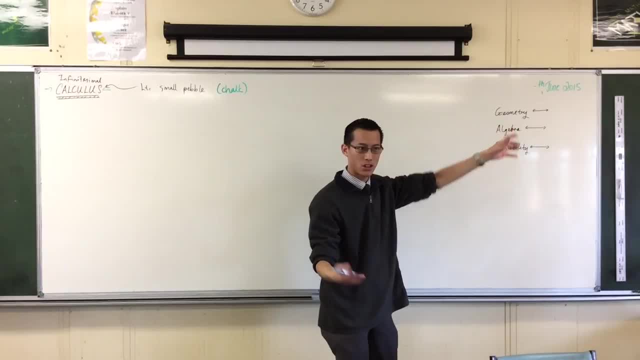 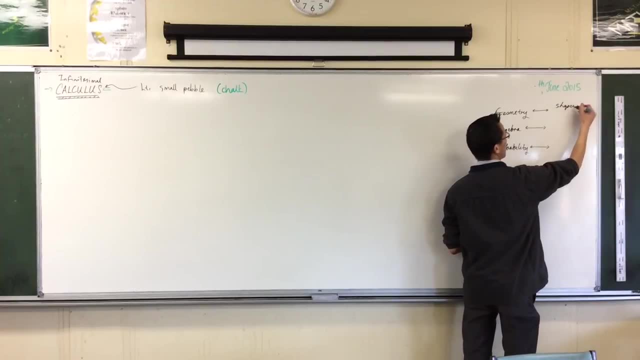 Geometry, for instance. we're familiar with geometry. When you think geometry, you think shapes- right, You think shapes things that take up space. right, Shapes planes and space right. That's what geometry is about, like dimensions and all that kind of thing. 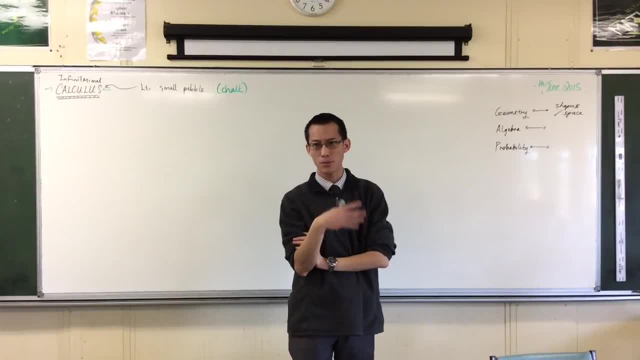 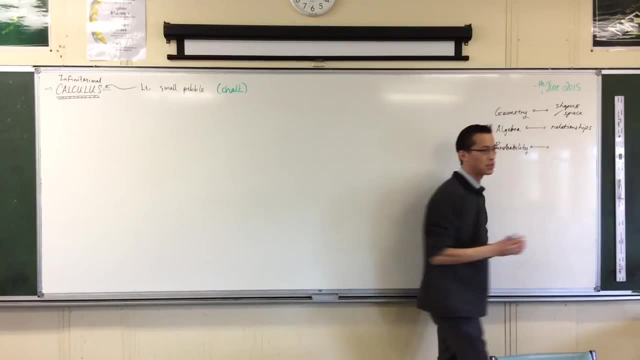 Algebra, this is a bit trickier, right, But all those x's and y's and pro-numers and unknowns. what they're really about is quantities that are related to each other, Things that change together in proportion to each other, in inverse proportion to each other, all those kinds of things. 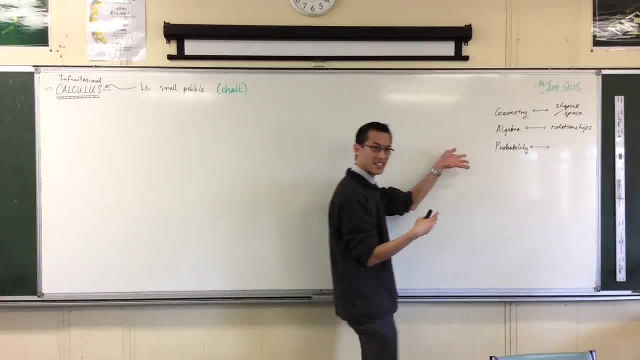 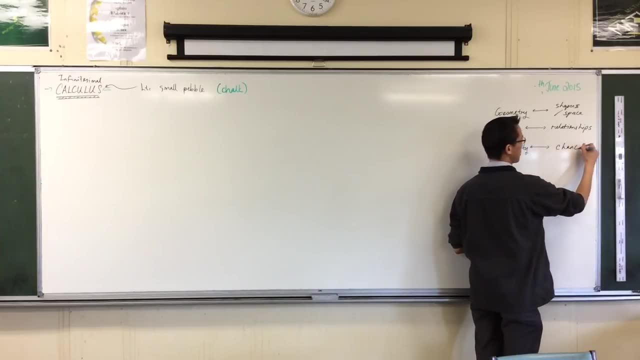 If they're related in algebra, it will help you understand it. Probability: that's a bit of an easier one. It's the mathematics of what Chance, uncertainty, right When you're like I'm not sure if something is going to happen, but I can know. 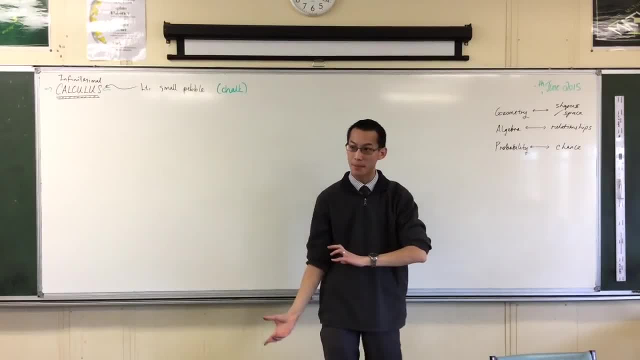 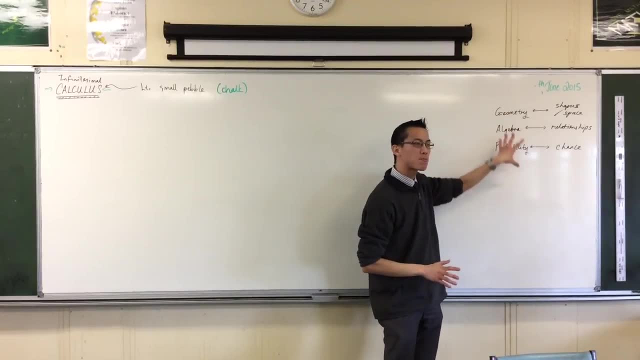 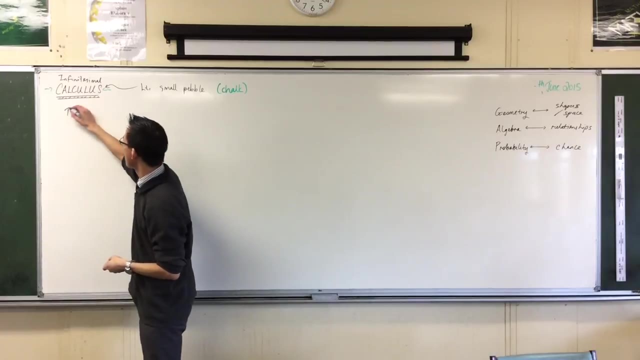 like the basics of like: this is more likely to happen, less likely to happen happen. am I going to win the lottery or not? am I going to get an A tariff of 99.05, etc. Each branch of mathematics has its key idea. Calculus is the mathematics of all things. 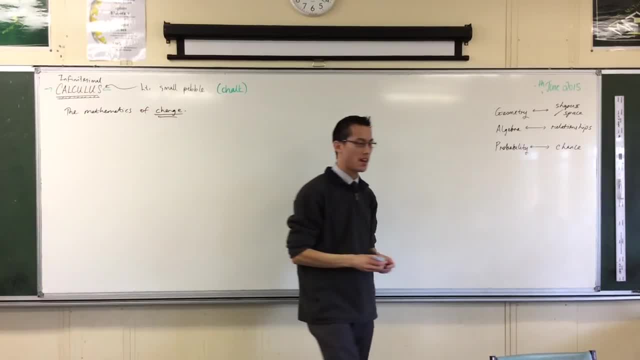 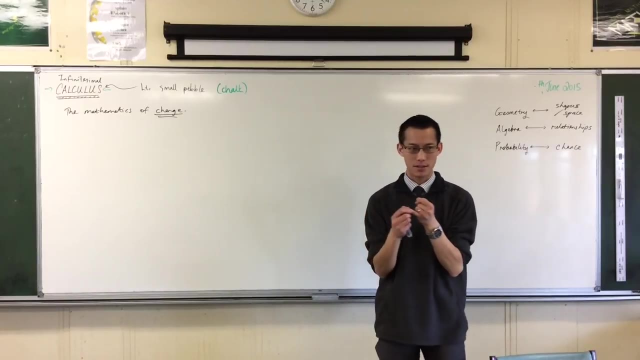 that change, All things that change, And you know what? There's lots of things in the world and in the universe that change. So you can kind of imagine why calculus kind of took over, In fact, number one, the preliminary NHSC courses that you're doing, mathematics. 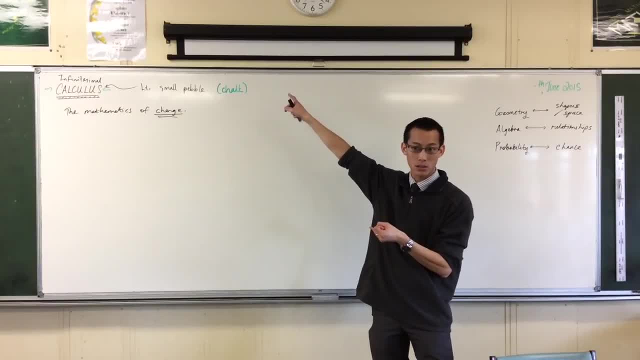 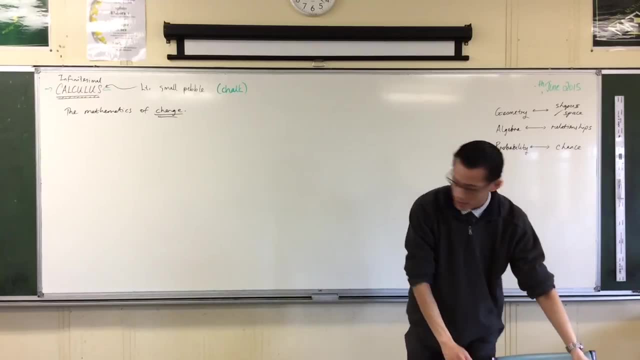 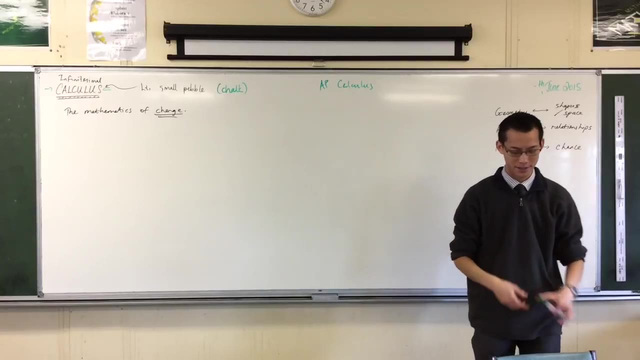 and mathematics extension one are called the calculus courses. They're a good 70-80% plus calculus and it's like sub-topics. In fact, the equivalent of what you guys are learning in America is called AP calculus. The AP stands for advanced placement. It's 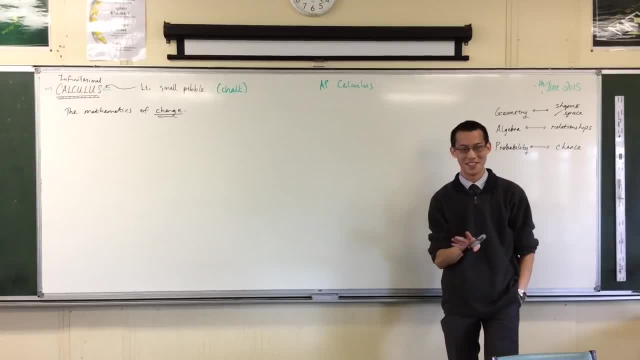 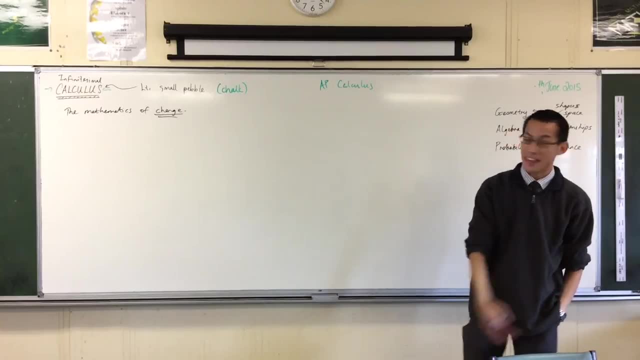 it means we're. you know you guys, we don't mess with you guys. you guys are serious about your maths. The course is called calculus, and in some ways so is ours. It's just not given to them. There's pre-calculus and then there's calculus. It's like: this is the things. 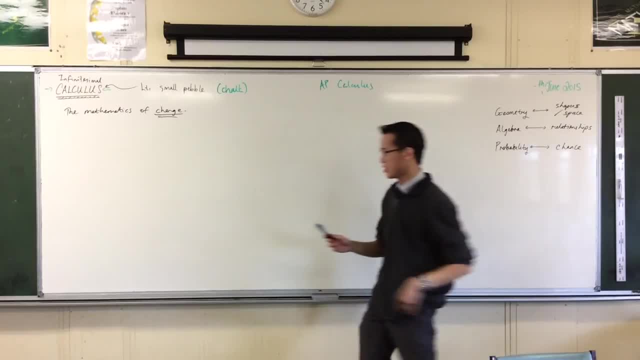 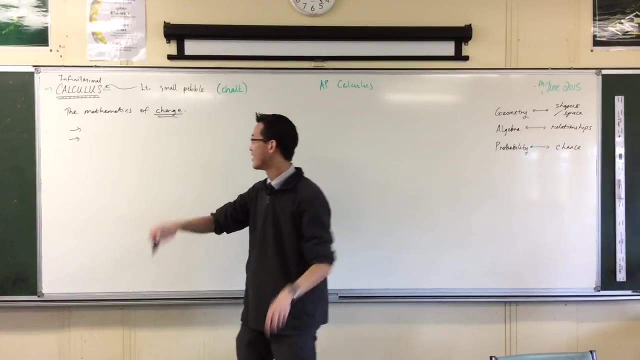 preparing you for this. Now, calculus, you need to know it was developed not jointly but independently by two guys in two countries at exactly the same time. There was a huge argument between these two As to who invented it. By the way, before it was called calculus, it was called the. 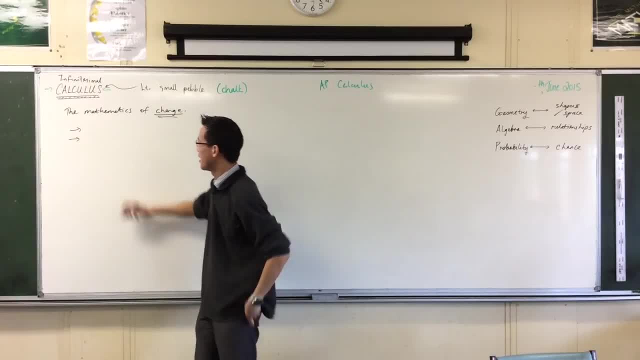 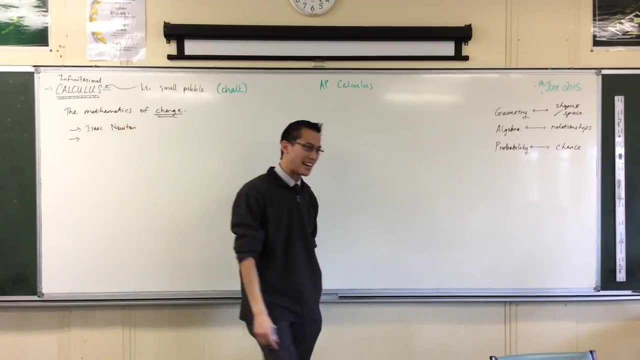 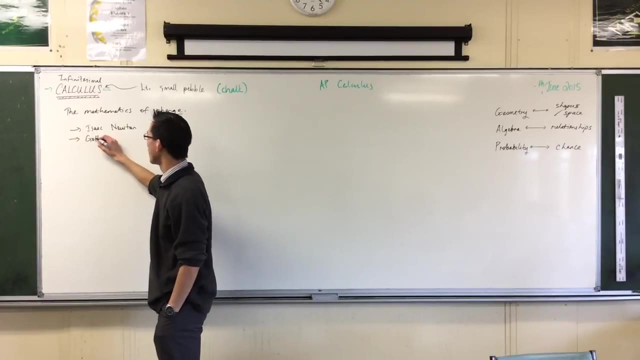 calculus. The B is like a, you know, capital C calculus. The two guys are one. you might have heard of a guy named Isaac Newton Guy in England, right, You might have heard of him. The other guy, the other guy you will probably not have heard of, Gottfried Leibniz. 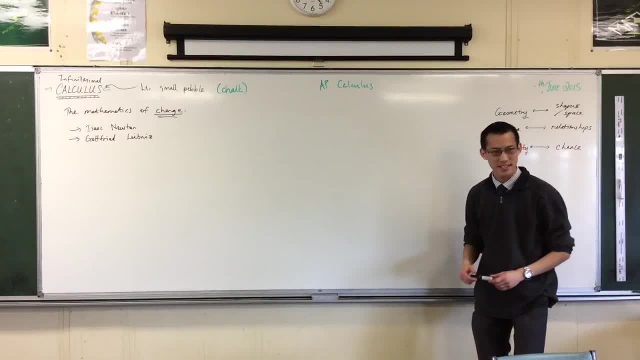 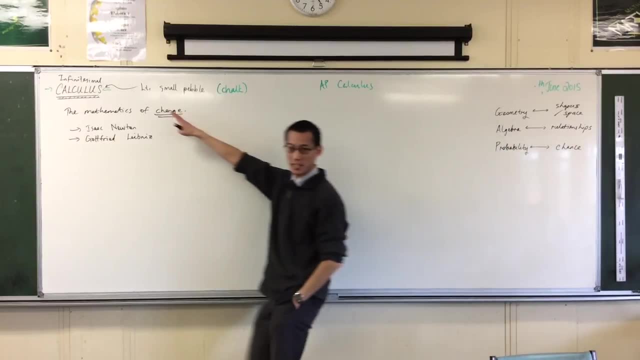 German guy, Newton in England, Leibniz in Germany, And both of them jointly- sorry, not jointly- simultaneously- developed this big idea. okay, And I'll tell you later on when we get to it. you can remind me why it's unusual that no one's heard of Leibniz and 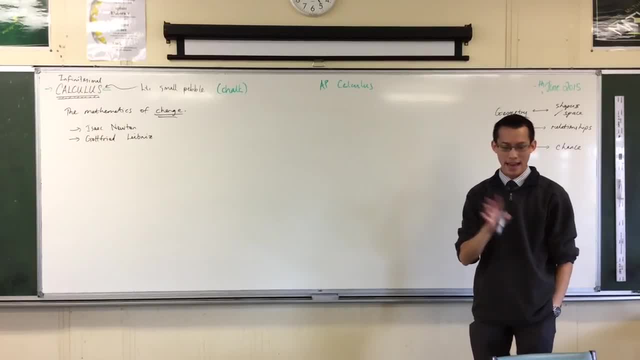 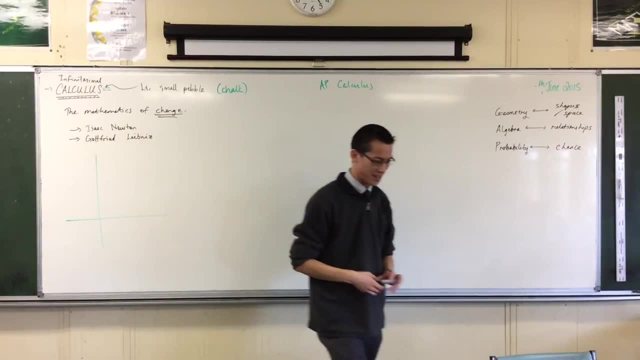 everyone's heard of Newton. okay, So here was the problem, and this is the famous part that we're each trying to work out, okay, So Newton? well, actually, yes, Newton was sitting under a tree, right? Or so the story goes: Newton was sitting under a tree, right. 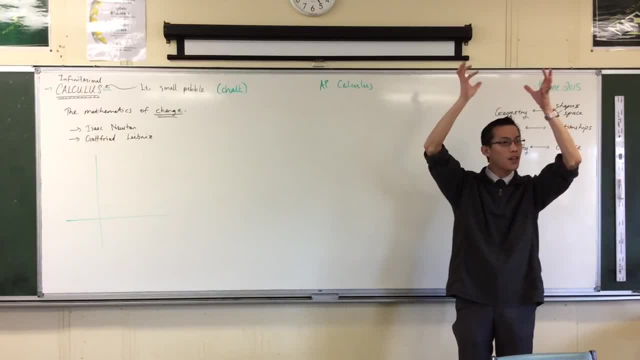 Or so the story goes. Newton was sitting under a tree, right, Or so the story goes, Newton. well, actually, yes, Newton was sitting under a tree- right Or so the story goes- And he saw the apple fall from the apple tree. It fell to the ground. 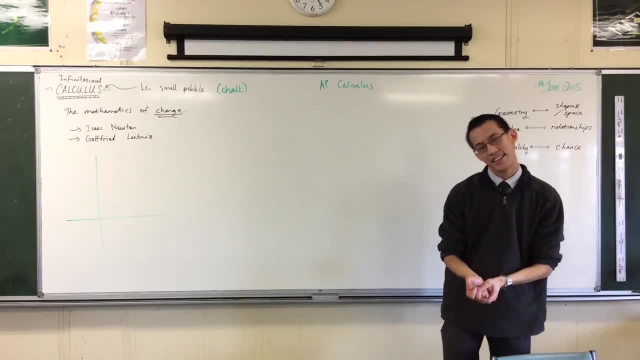 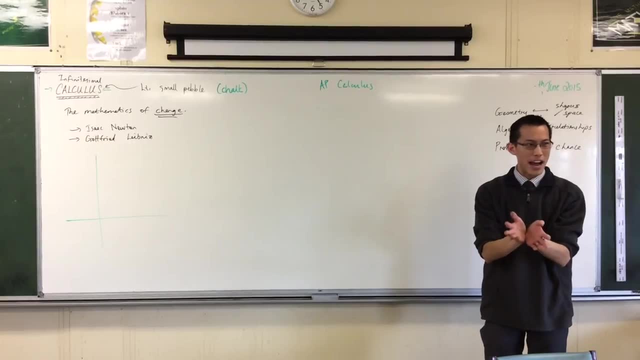 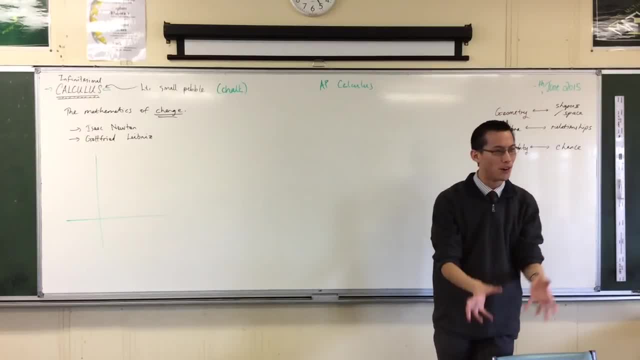 was an actual apple or not is up to debate, But the point was that he watched the apple fall and he watched it fall to the ground and he's like, oh okay, Gravity, Gravity's a thing, It makes the apple fall. 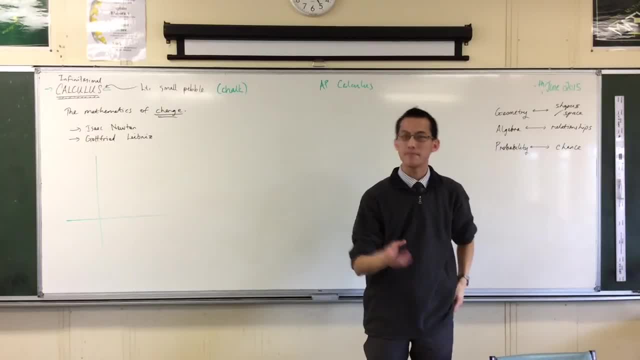 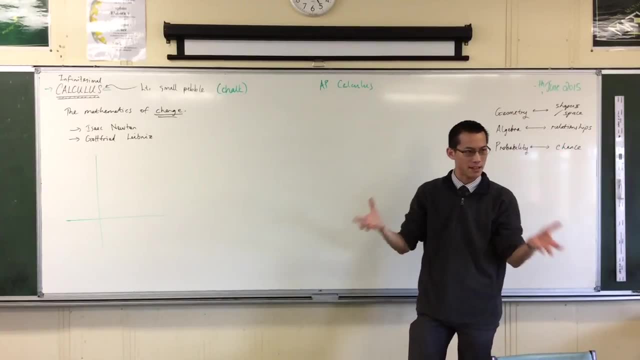 It makes the apple fall. But then, as he watched the apple fall, he thought the moon is way up there right And it's also being held in place by the same thing that makes the apple fall right- Gravity- But it doesn't hit the earth. Why does it not do that? Why? 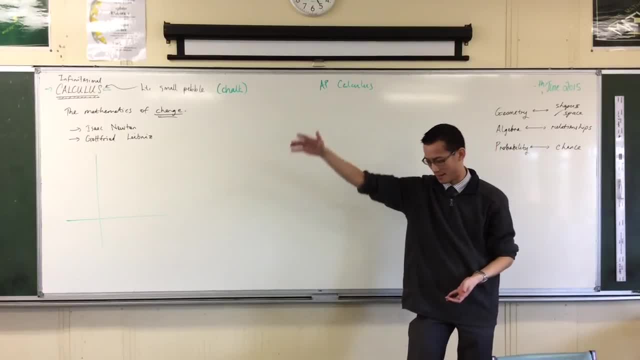 does gravity do this to this object, but that object just stays way up there And he's like: how do I work this out? So what he did was try, as we've been doing, To take a problem which you don't know how to phrase and turn it into a problem which 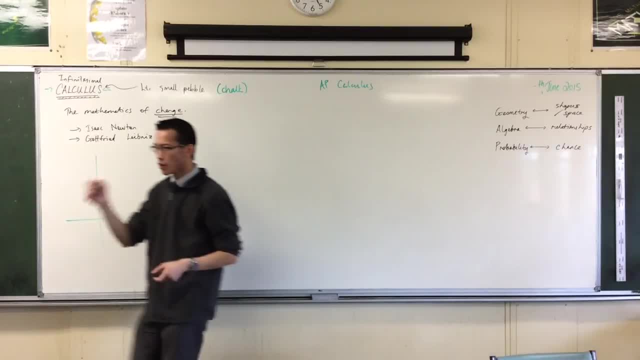 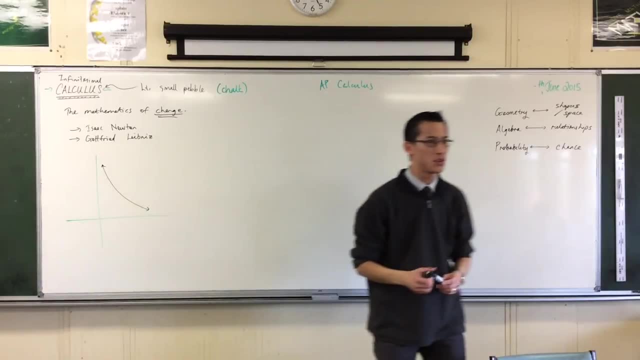 you can phrase, because then you can solve it. He ran into a problem. Gravity does something unusual. It does something like this: Gravity, like most forces in the universe, is inversely proportional. The force that it exerts on something is inversely proportional, based on the- I was going to say the distance, but 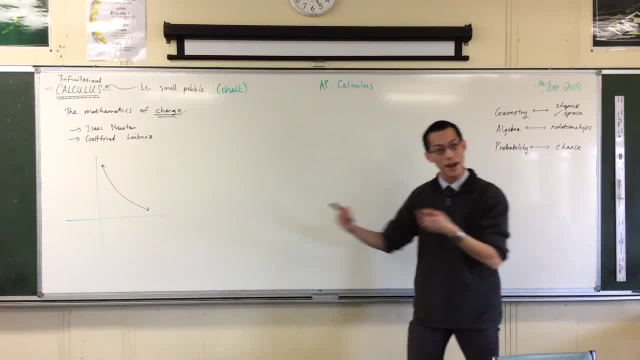 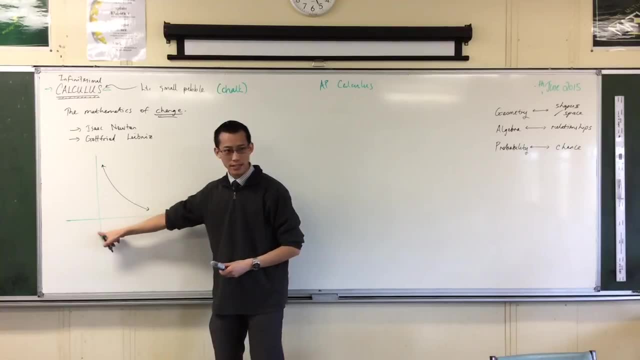 it's really the square of the distance that you are away from something. Okay, So, the further away you get from something. So if I have over here, distance, Distance, Distance, Distance, Distance, right As your distance increases the force of gravity, and well, actually everything, 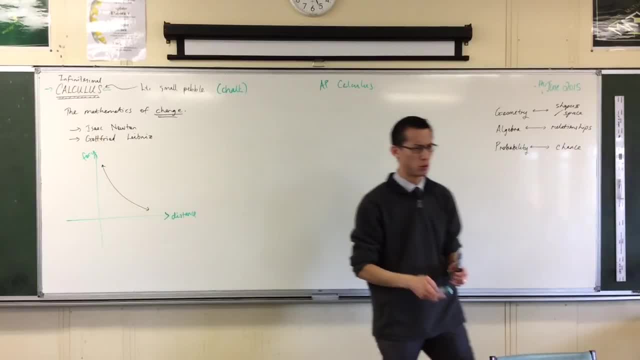 really, If you think of the electrostatic force- it's Coulomb's law, I think- It gets smaller and smaller and smaller and it drops off like this: Okay, It drops off quite fast. Okay, Now here was his problem. right, He was trying to work out. okay, how do these things relate? 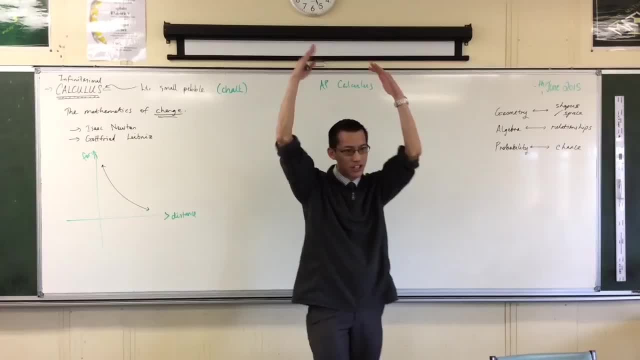 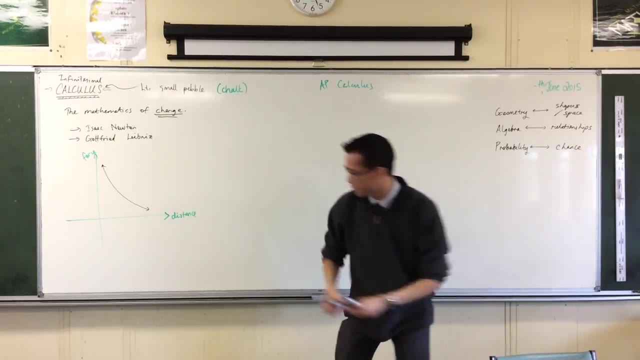 to each other. How does gravity change over distance? Right, This is the problem he was to solve. and this is tricky because this thing, this thing is changing at different rates everywhere that you look, right. for example, if you just compare it with a straight line, you can draw one of these for me. okay, 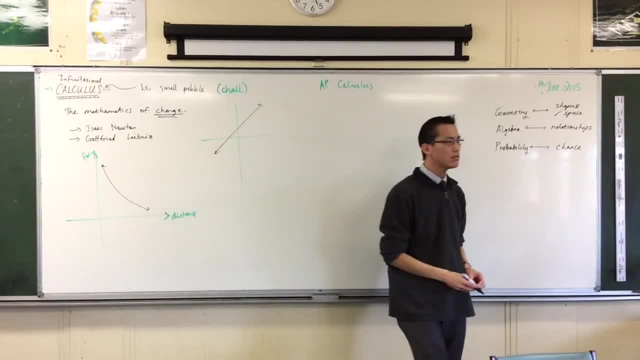 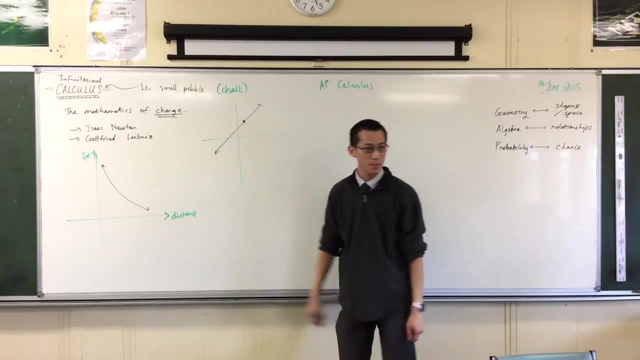 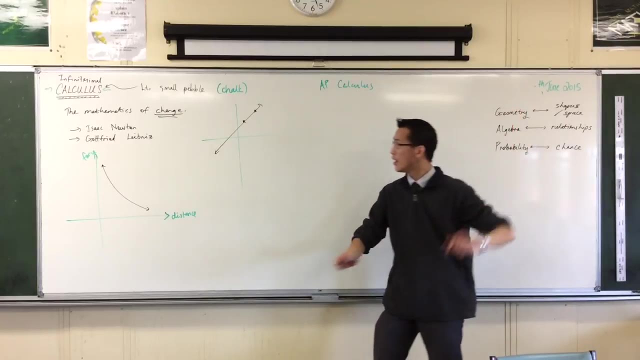 go straight line. if you want to know how this straight line is changing. okay, that's not hard to work out. that's not hard to work out. you just think, for example, at a particular point in distance or time, whatever value, you compare it to another point. okay, and if you've got two points on there, you can. 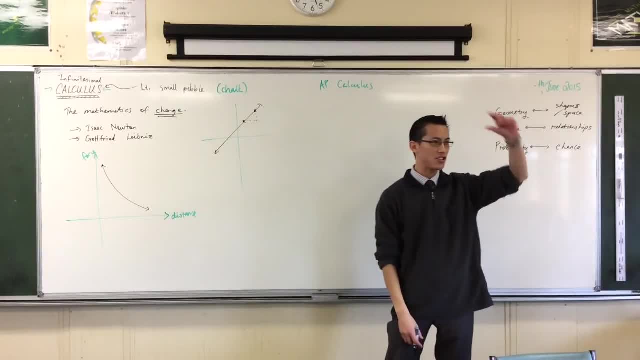 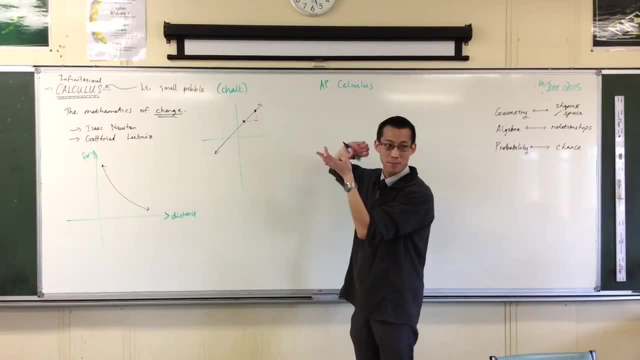 just say: look, I'll just compare how much it changes in one quantity versus how much it changes in the other. you just get them as a ratio right. we know that nature ratio by the name starts with a G gradient. right on a um, on a Cartesian plane, you'd say, look, this is vertical, so you call that rise and this is. 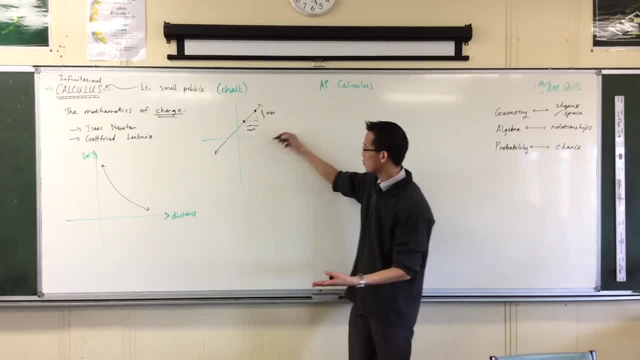 horizontal, we call that run, okay, and the gradient, which it's M, still who knows why. okay, the gradient is just the ratio between those two thing. okay, but there's a problem here. there's a problem here: no matter which two points you pick, you're always going to get a different value. see the thing about this, the reason why. 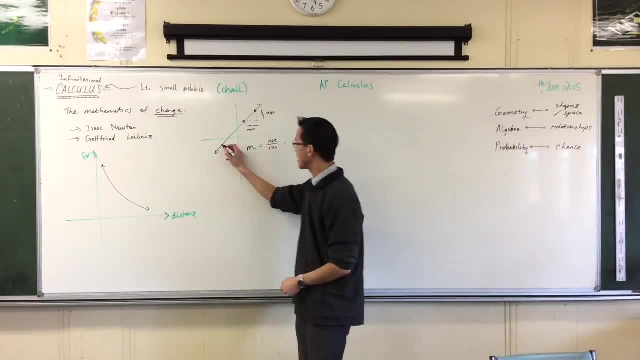 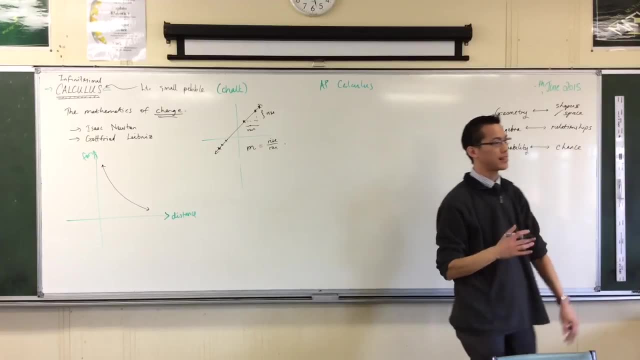 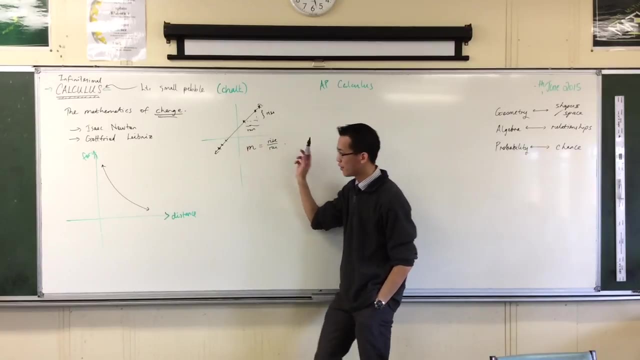 this works is because I can calculate that, or I can calculate between these two points, or I can calculate between these two points, and you're always going to get the same value. you always get the same gradient. it's gonna be this constant right. we know how to read that off, but here we have some trouble you. 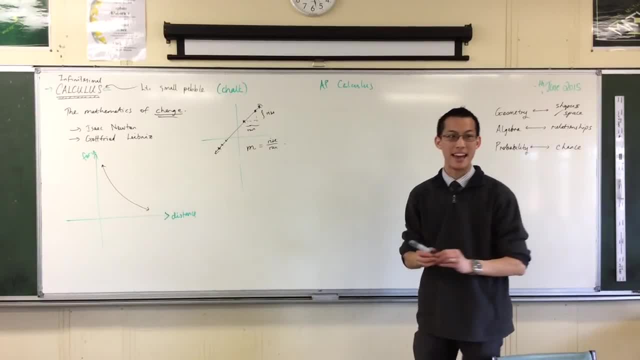 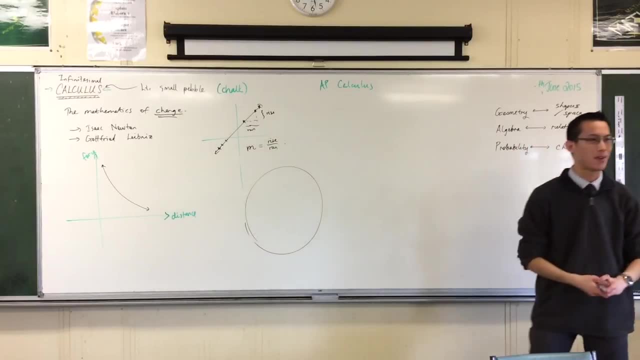 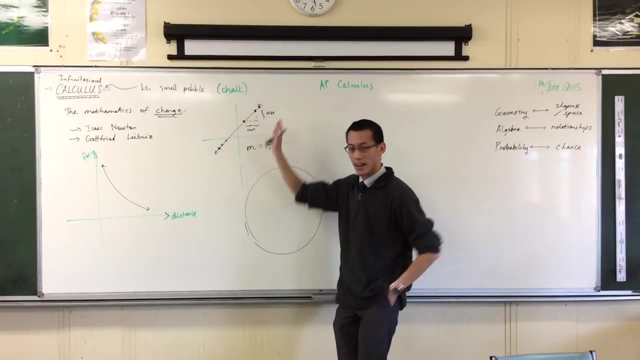 have some trouble. so here is what Newton did and it's ingenious. okay, think about, think about a circle. okay, yeah, I've done better, all right now. what he really wanted was: how much? how much am I changing it every any given point right now by grading? you guys already know in terms of like geometry, like what does. 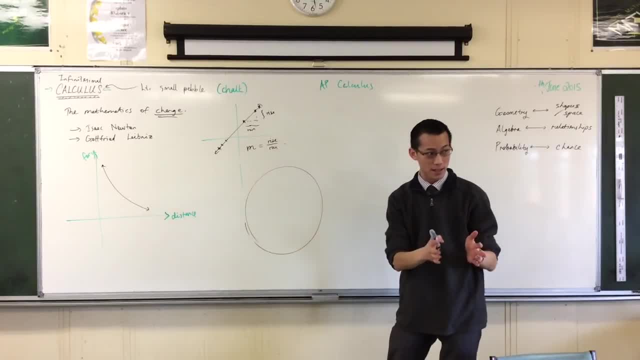 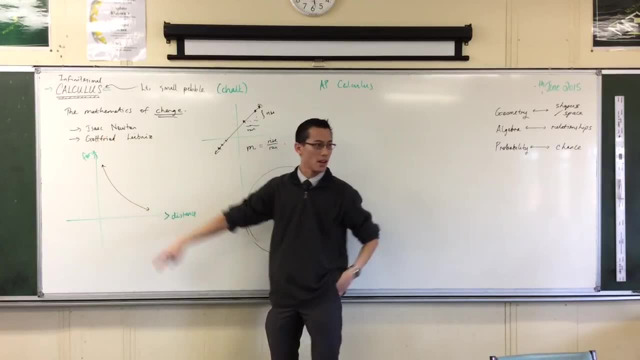 that look like it's the steepness of the graph, right? if you can know how steep something is at a given point, that's its gradient, okay. so he wanted to know, like I know, obviously it's steep over here and it's not so steep over here, but how? 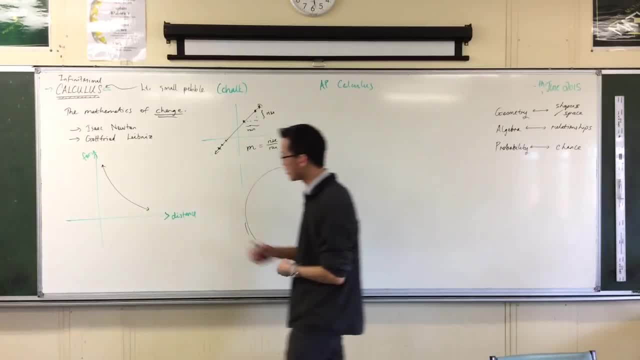 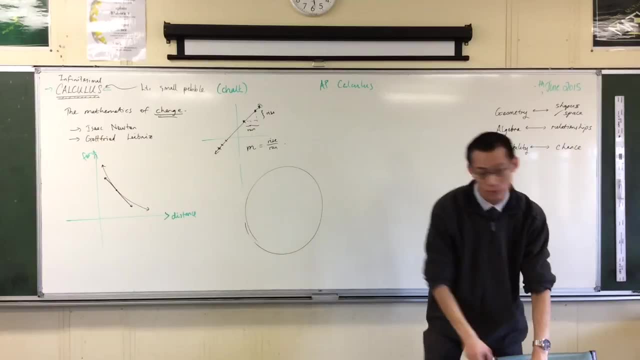 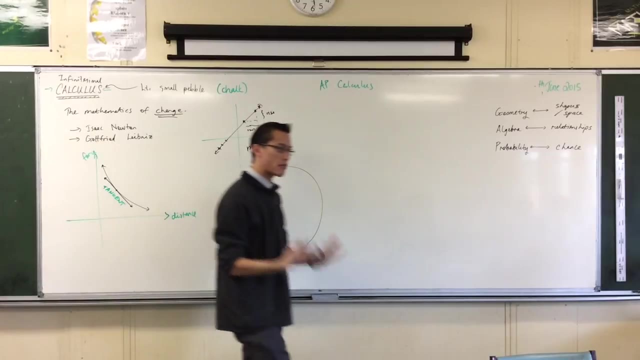 much okay. so what he was really after- the quantity he was after- was the gradient of the tangent. okay, this is a really critical idea: the gradient of a tangent. the problem with working out the gradient of a tangent is that gradient is rise over run. you have to have some run. you have to have two points. 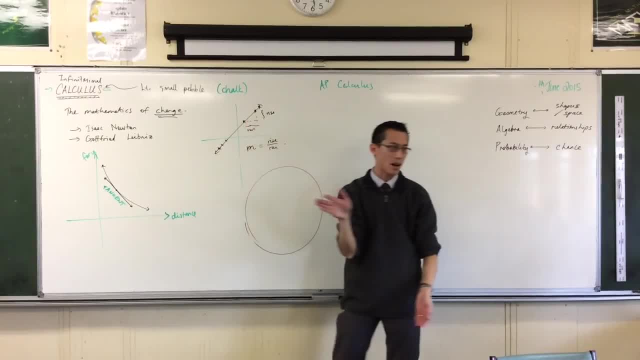 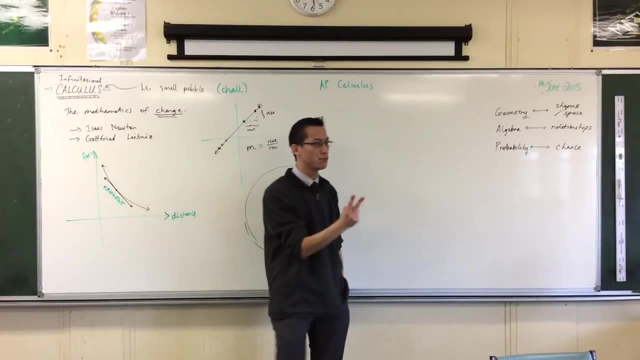 right to compare between y 2 minus y 1 over X 2 minus X 1. you need a y 2 and X 2, but a tangent, by definition, doesn't have two points. it's just got one right, in fact. that's why it's the word tangent. does anyone know? just like all of this? 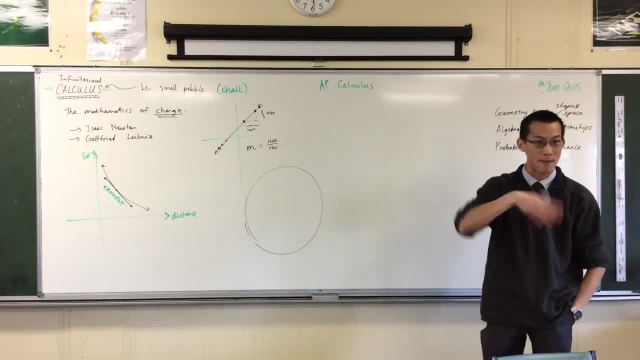 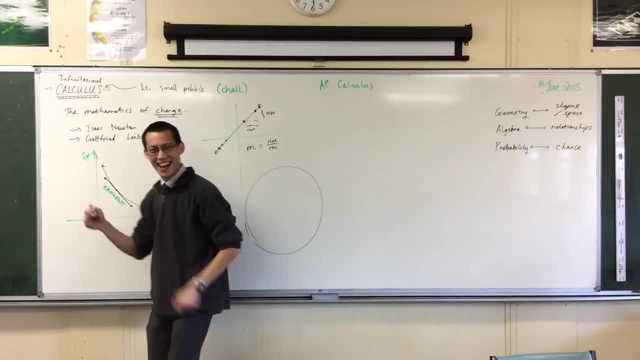 right. we have another way: English language, which comes from the same route. we don't know what it is. they use it very often: tanguy. well, what does a ẕ Yasmeed conventional yet think of 21? What does tangible mean? It means you can touch it. 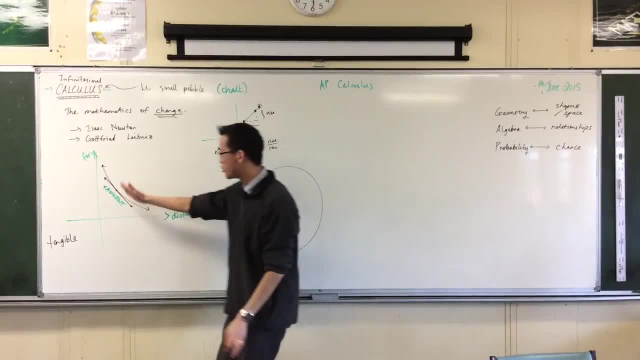 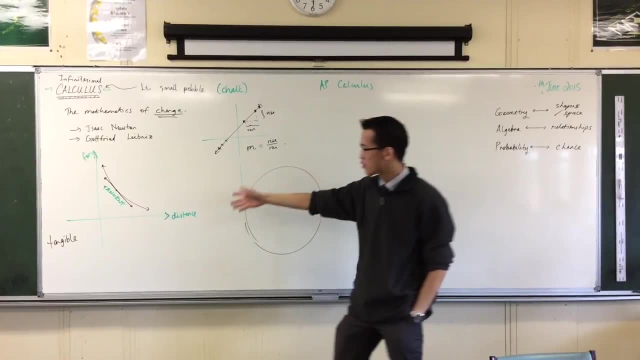 You can touch it right. So a tangent is something which just touches One point. So this presents problems for us and Newton and Leibniz trying to work out what's the gradient at that point, Because there are no two points to compare by definition. So here's what they both do.